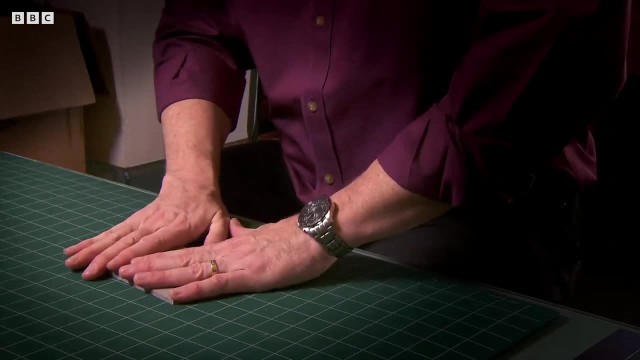 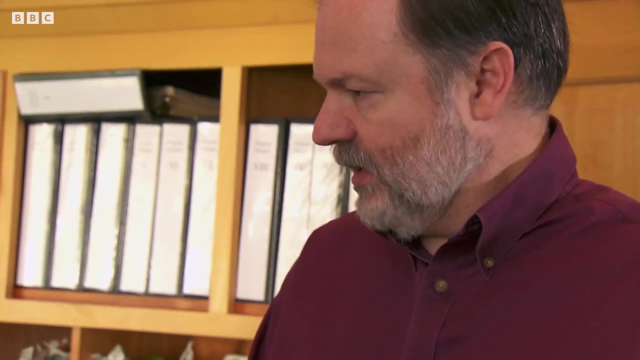 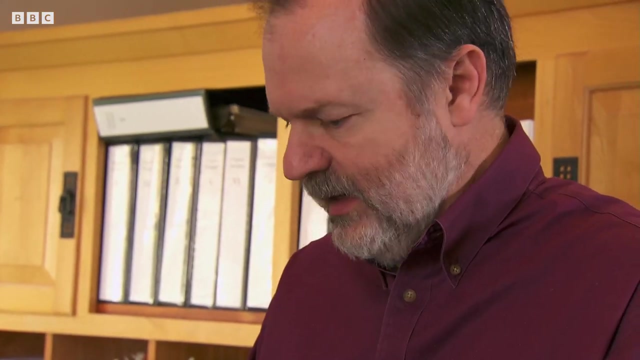 small. This is the pattern that I just folded. It's called a Miura Ori and it was discovered by Koryo Miura, a Japanese engineer working in the Japanese space program. He was studying the way thin plates buckle under stress, and that led him to discover this fold pattern. 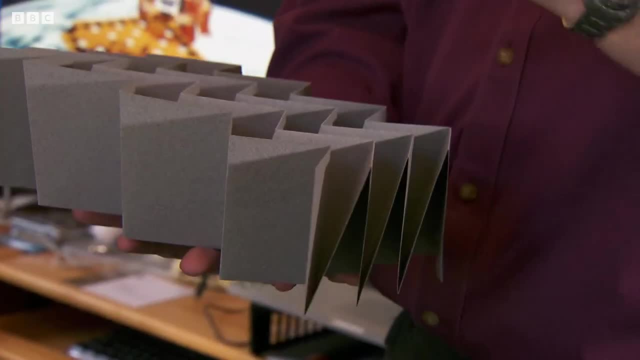 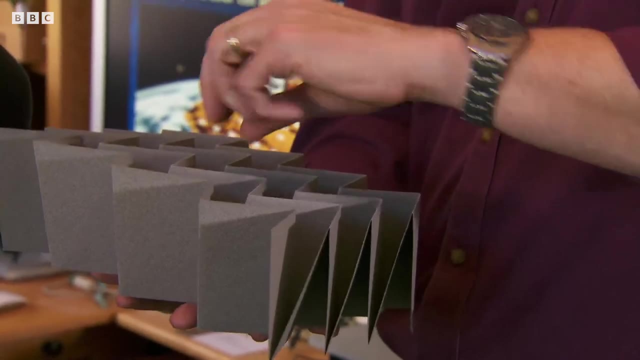 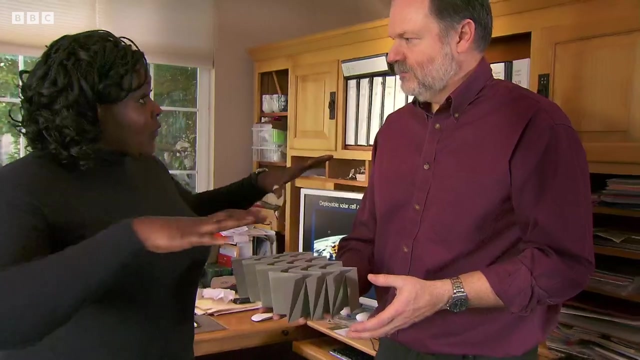 And he explored it and found it had a really nice property: It opens and closes with all of the folds happening together because they're mechanically linked. Then you would only need to bend a single fold to make the entire structure open and close. So when you open one fold, all the other folds follow and actually flatten out. 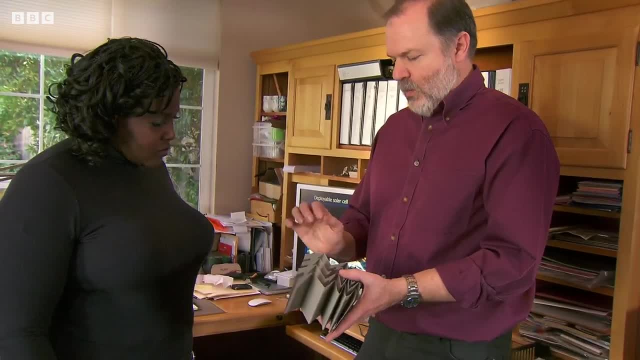 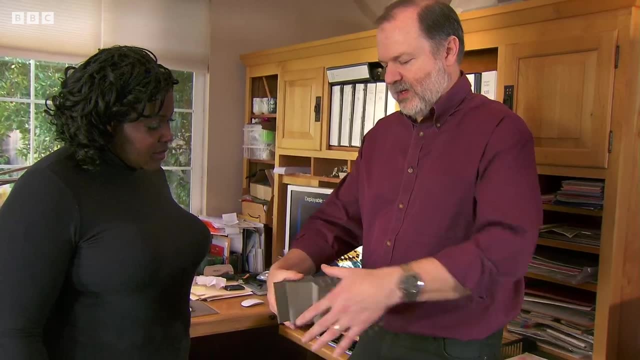 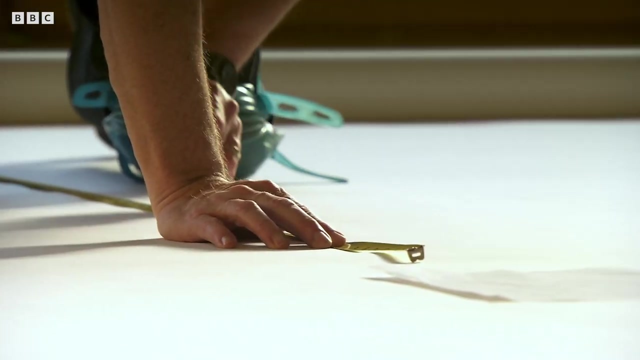 So if this were a solar array in space, you'd only need to put one solenoid or mechanical mechanism on one fold, and that fold would be enough to make the whole thing open up. Robert offers to show me how to make something the size of a solar panel. 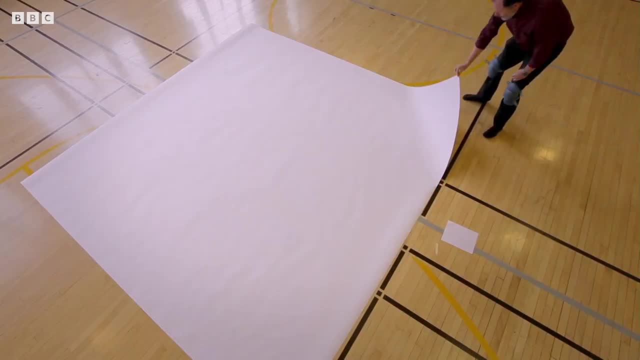 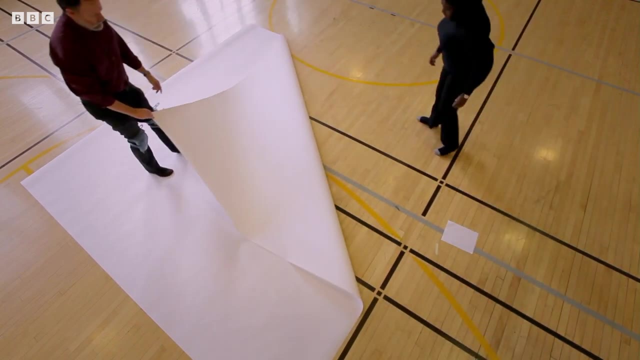 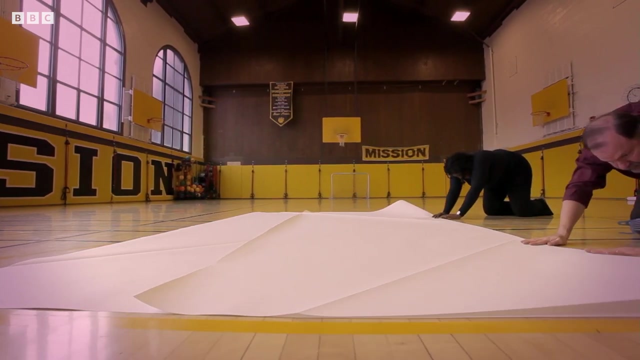 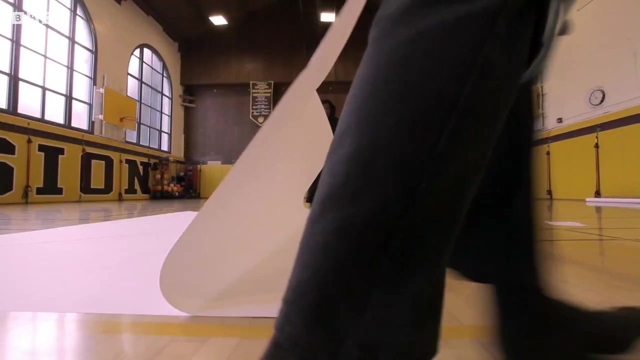 Yes, A solar panel fit into a small payload bay. The sheet is nine square metres and its transformation will involve 72 separate folds. Robert pre-creases the folds to increase accuracy and flexibility. Wow, Wow, they're forming a spiral. 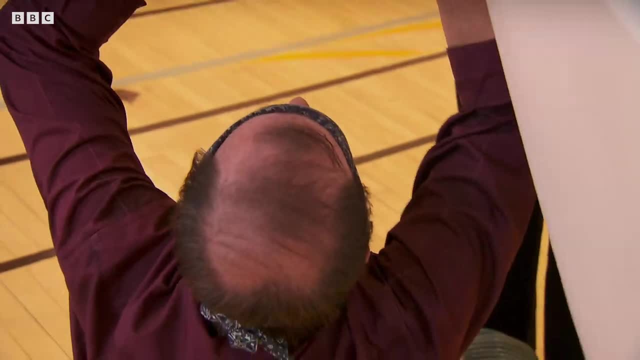 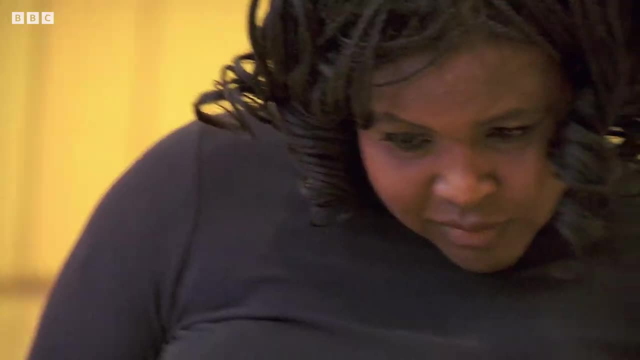 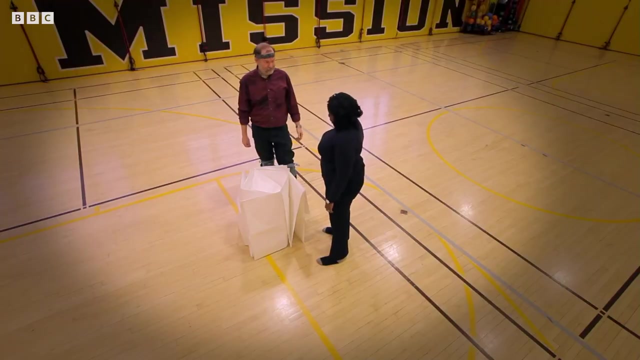 Yep, Origami may be Japanese, but I never expected it to be a martial art. It certainly needs one or two ninja moves, All right. So you've taken that huge piece of paper and reduced it to this. That's right. So if this had been a solar array, we've taken it down to the size. it could go into a rocket. It goes up in space, opens up and then it's ready to deploy back to its original flat state. We've gone down by just about a factor of 100, about 10 in each linear dimension. 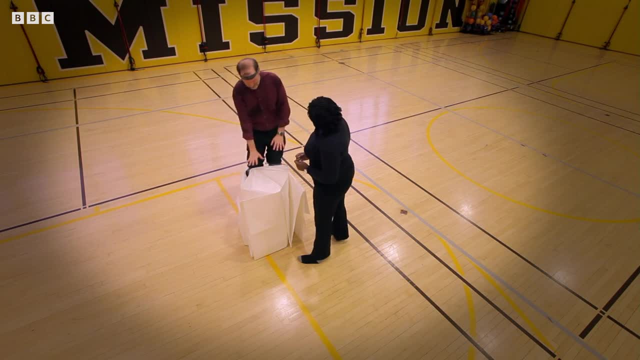 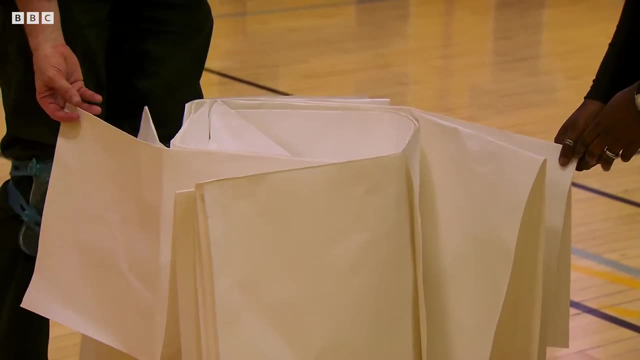 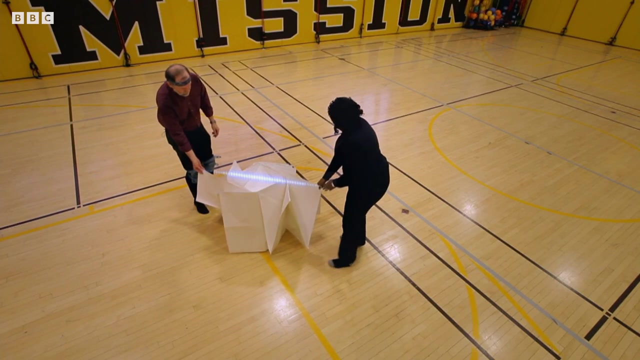 And, of course, we got that by going from completely flat to a vertical tube like this. Yes, but much easier to stow in a rocket, Exactly. Robert's creation is clever enough, but the real revelation comes with its opening, Although the design appears complex.